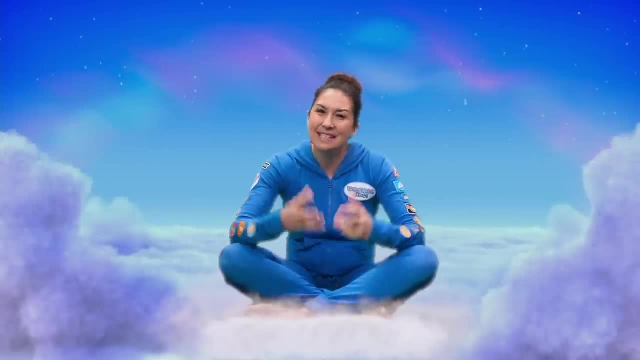 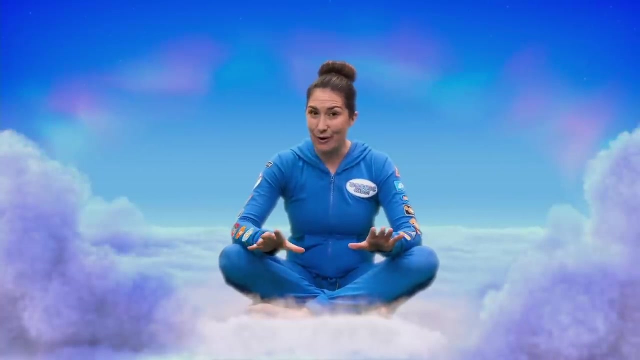 listen to each other properly. This means we're better at looking after ourselves, at making sure we get what we need, and we're able to notice when something just isn't quite right and it needs fixing. Okay, let's do a body scan now. It doesn't take very long and it feels great. 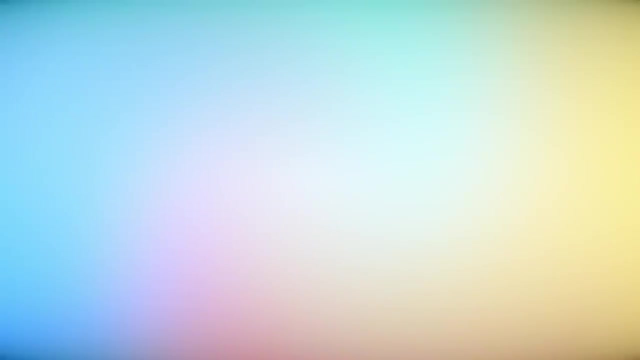 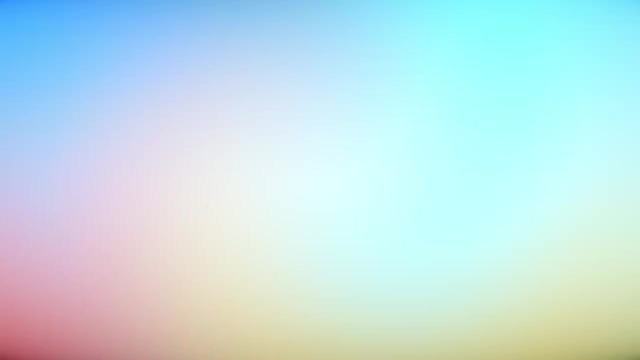 Okay, let's do a body scan now. It doesn't take very long and it feels great. Okay, let's do a body scan now. It doesn't take very long and it feels great. Let's move up the body now and check in with your legs. 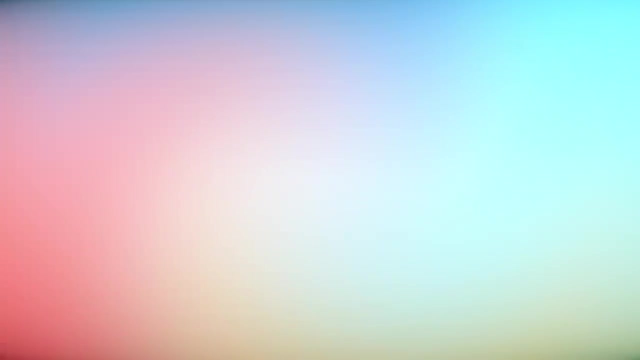 Go nice and slow Your ankles first. Move your attention to your ankles. Now up your lower legs, Your calves, the backs of your lower legs, Your shins, the front part of your lower legs, Notice your knees. Any sensations there? 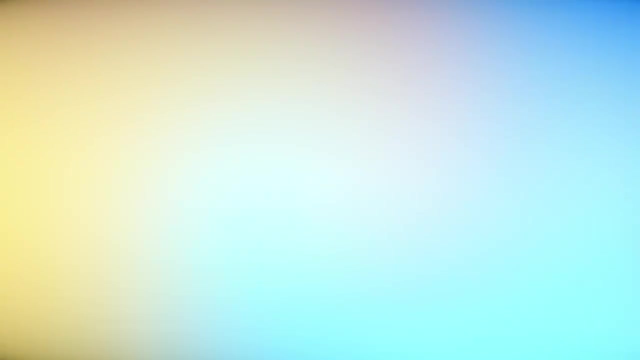 Now your upper legs. Notice the legs, the top part, your thighs, the top part of your thighs, and now the backs of your thighs, the sides of your thighs. Notice all the sensations, Whether your legs are tense or relaxed. Are you holding on anywhere in your legs? 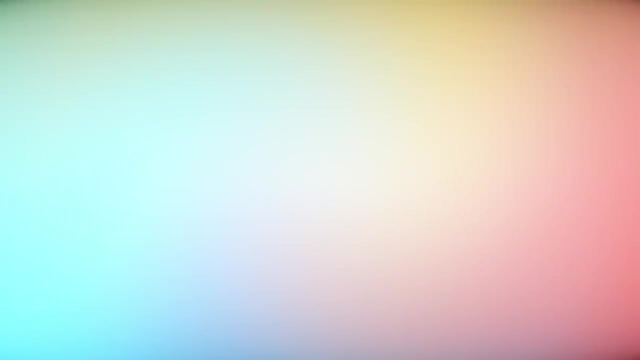 Can you let go? Are you warm or cool in your legs? Can you feel the weight of them? Breathe here, keeping your attention on your legs, Just noticing, just sensing. Now come up to the middle part of your body. 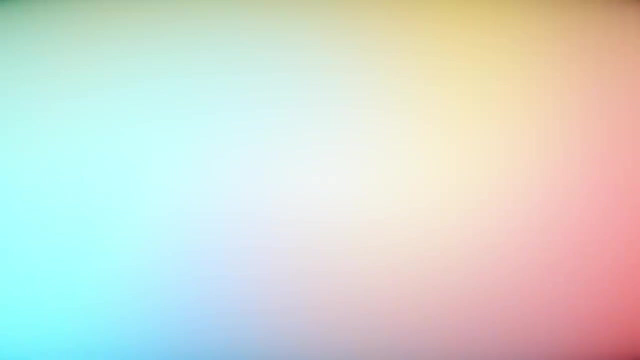 Your tummy. Notice the sensations there in your tummy. Your chest, Moving your attention up to your chest. The sides of your body Where your ribcage is, Your shoulders, Your shoulders, Your shoulders. Notice all the sensations there in the middle of your body. 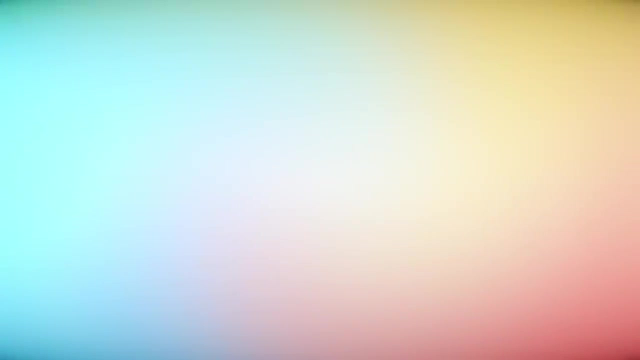 And move that attention round to your back. Can you feel anything there? Feel the weight of each part, Notice the warmth, The heat, Any sensations, Any tingling, How your body feels here, right now. Keep your attention here, on the middle of your body. 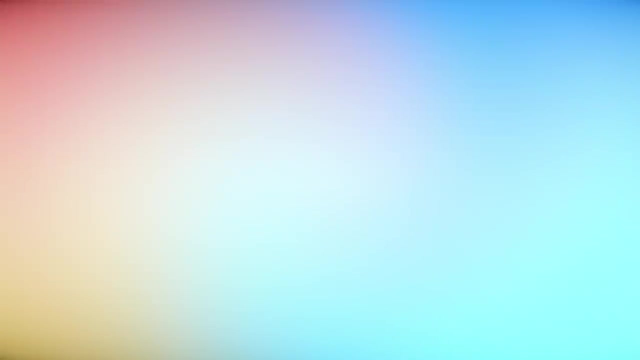 and breathe into all that you feel. I feel a subtle tingling in mine. What are you feeling Now? scan down through your arms, Your arms, Your upper arms, Noticing the sensations around your shoulders, The tops of your arms. 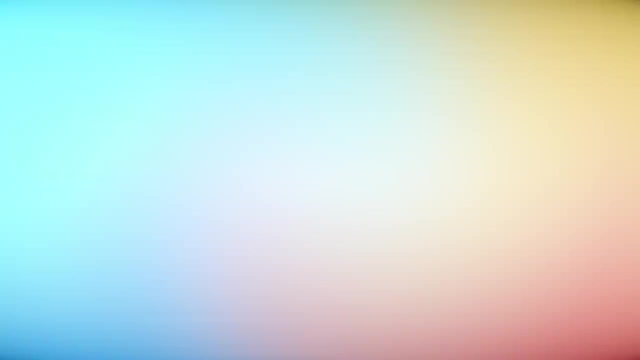 And now scan down to your elbows And your forearms, The back and the front. And now scan down into your hands, Right down through your fingers, Your thumbs, Each one, Slowly scanning each part And just noticing what's there. 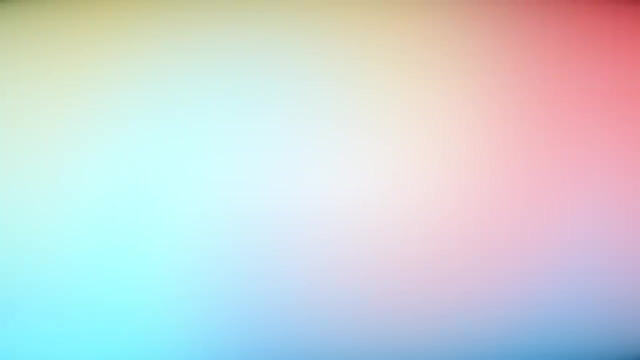 What's there? Is there warmth? Is it cool? Maybe some lightness Or tension, Any tingles, A sense of heaviness? maybe Let them be what they are. No need to change anything, You're just noticing Learning. 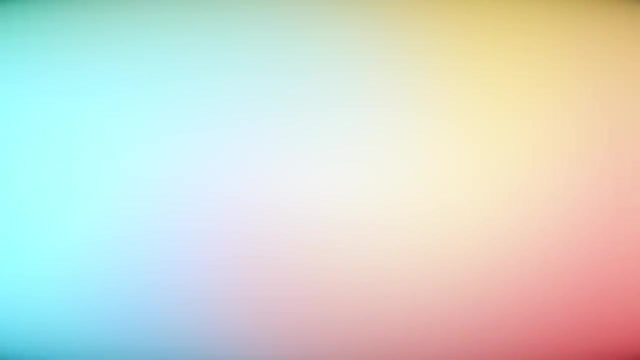 Helping your mind and your body to be friends, Allowing everything to just be Whatever is there, Whether it's nice, pleasant, or it's challenging. maybe Just let it be. You're logging it all, Breathing here, Noticing your arms. 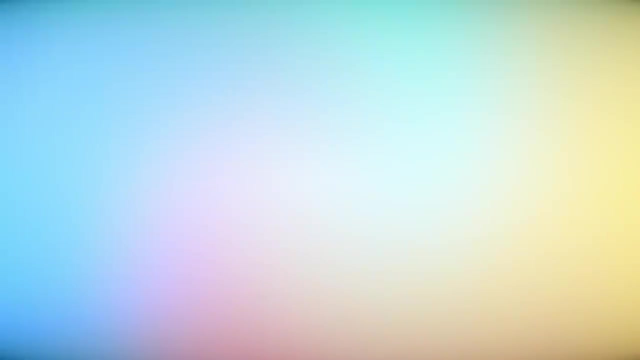 Lastly, take your scan up to your neck. Notice your neck, The sensations inside and outside. What can you feel? Move that attention to your head, Feel the weight of your head on the floor, Sense any warmth or coolness. Notice your face. 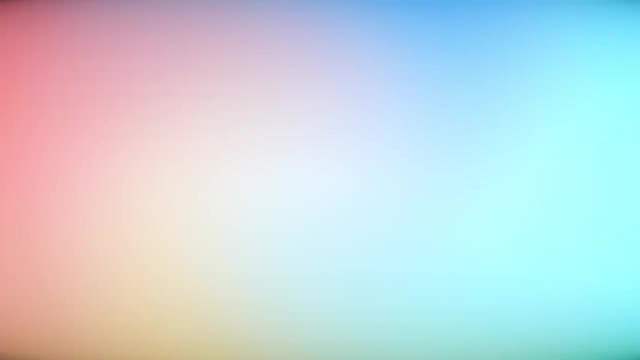 Notice your face, your jaw, the sides of your face, just in front of your ears. Notice your tongue in your mouth, your lips, your chin. Now scan your eyes. Notice your eyes And even go behind your eyes. Breathe here.